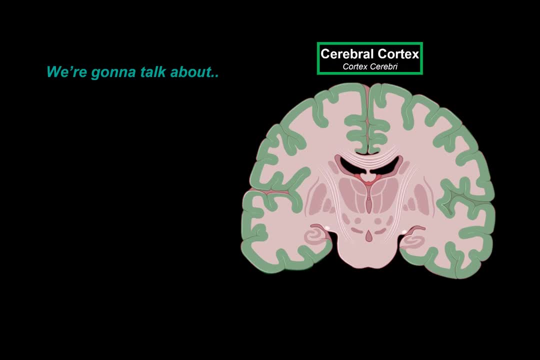 So again, the cerebral cortex is what we're going to focus on today. So in this video, we're first going to look at the functions of the cortex, Then we're going to go through the different surfaces and fissures. While doing so, we'll go through the dural septae, because they're located within the 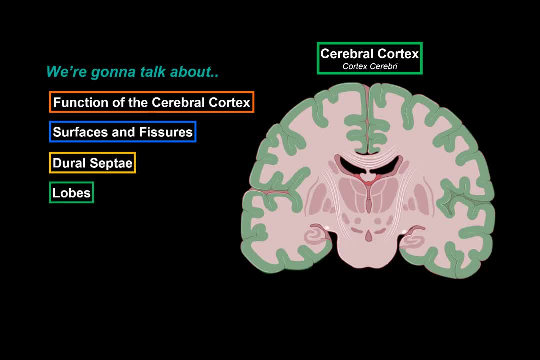 fissures of the brain. After that we're going to go through all the sulci and giri associated with each lobe And then in the next video we're going to talk about the rest of the pallium, which is the white matter of the brain and the basal ganglia. 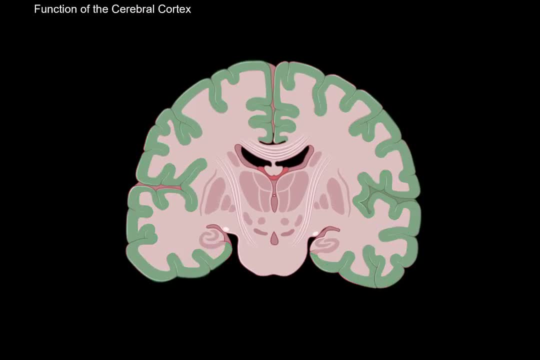 So the cerebral cortex is a highly folded sheet of neurons which have a thickness of around 1.5 to 5 mm. So the cerebral cortex is a highly folded sheet of neurons which have a thickness of around 1.5 to 5 mm. 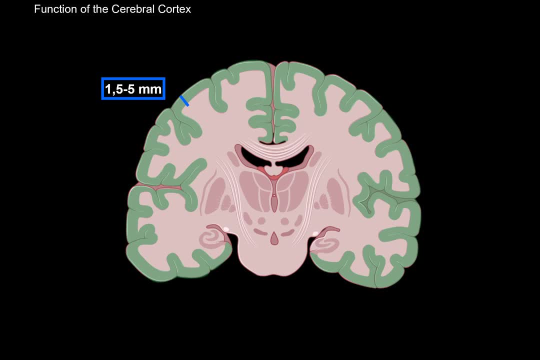 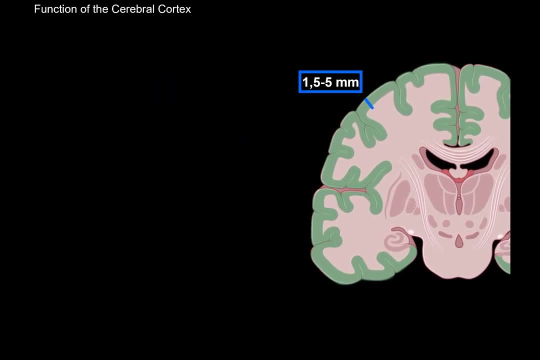 Depending on the region you're measuring. Now, why do you think the cerebral cortex differ in thickness along different regions? Well, to understand that, we need to have a basic understanding of the cortex layers. So if we take a small sample of it and look at it underneath the microscope, you'll 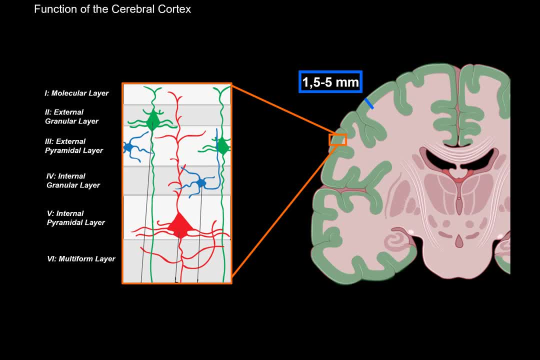 see 6 distinct layers, The molecular layer being the most superficial one, Then the external granular layer, External pyramidal, Internal granular And internal pyramidal, And then the multifoam layer. The thickness of the cortex varies because these layers differ in thickness depending. 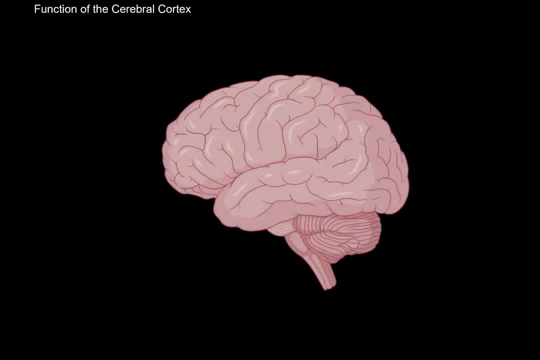 on the functions of the specific area we're looking at. For example, we've got areas in the cerebral cortex we call sensory areas that receive sensory information from the body. The primary somatosensory cortex receives information regarding somatic sensation. These sensations detect things like touch, pain, temperature and proprioception. 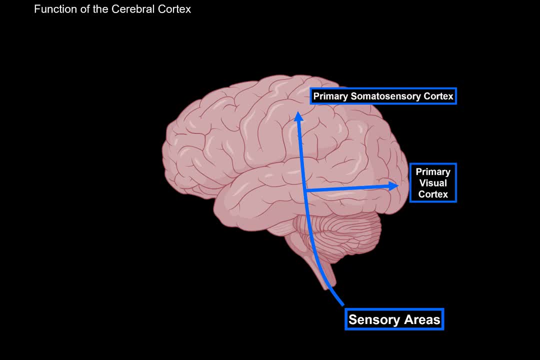 We have the primary visual cortex, which receives visual sensation through the optic nerve. We've got the primary auditory cortex, which receives auditory information through the cochlear nerve. Through an MRI, in general you will see that the sensory cortical areas are thinner on. 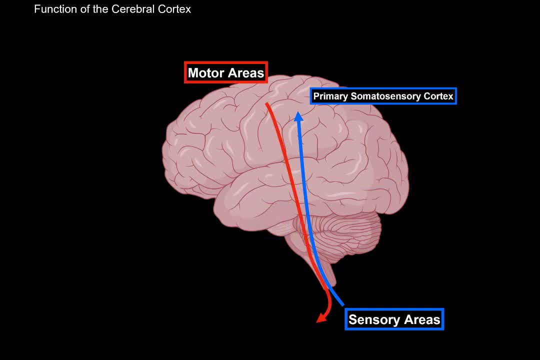 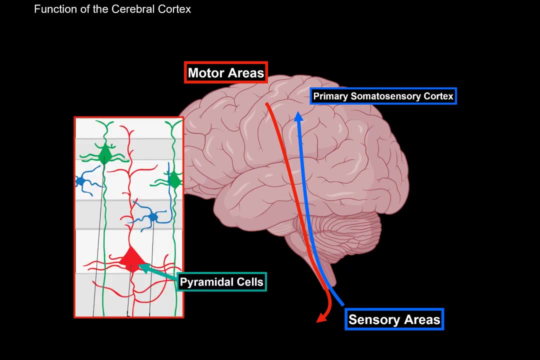 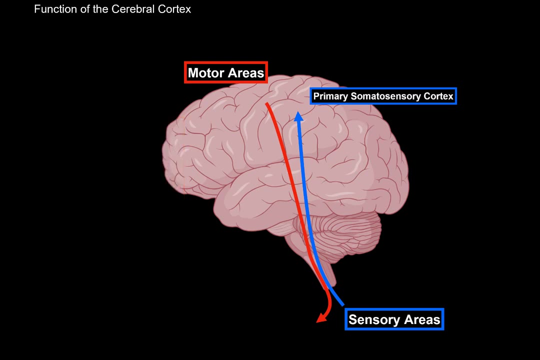 average, while the motor cortical areas, specifically the primary motor cortex, are generally thicker, And that is because the internal pyramidal layer has a denser amount of pyramidal cells, which are the ones sending down motor pyramids. We also have pyramidal tracts like the corticospinal tract and the corticonuclear tract. 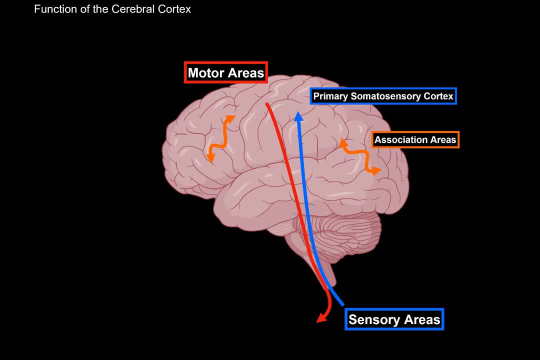 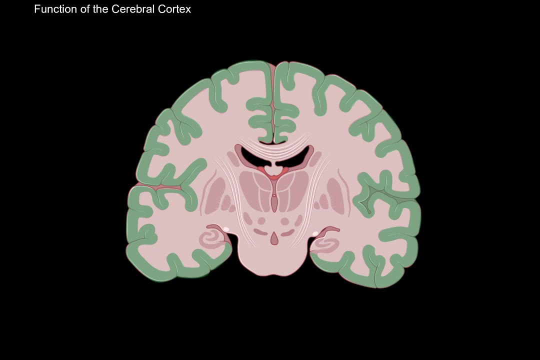 Between all the primary areas of the brain we've got association areas that interpret information from the primary sensory areas And based on that interpretation we react and communicate. So in general, everything that goes through the cerebral cortex is conscious. Everything that does not go through your cortex is subconscious. 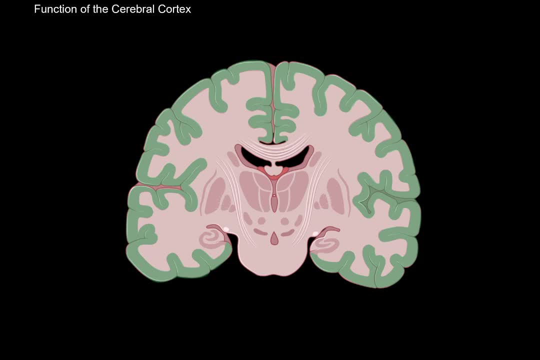 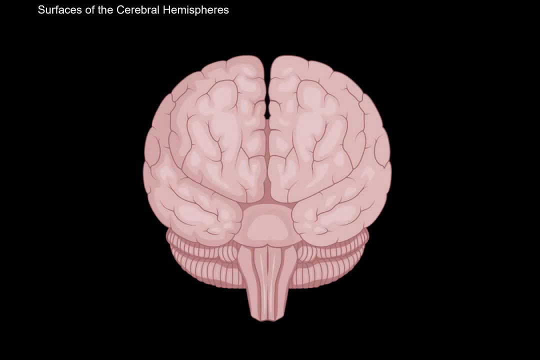 And that is the general function of the cerebral cortex. Now We've got two hemispheres, The left hemisphere and the right hemisphere, And this is what the surfaces of these hemispheres look like. So let's talk about that a little bit. 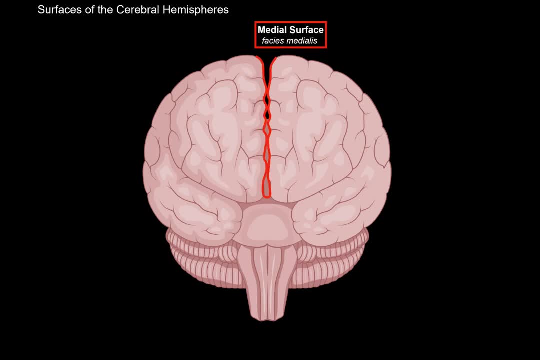 Each cerebral hemisphere has three surfaces. They have a medial surface facing each other, an inferior surface that faces the cerebellum and a superior lateral surface, which is the largest surface of each hemisphere. So these are the surfaces, But we also have large fissures here in this area. 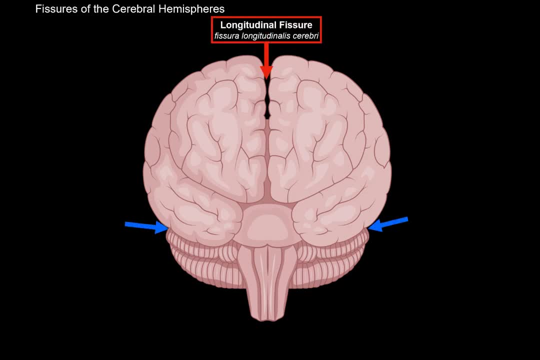 We have one right here called the longitudinal fissure, And these two between the cerebrum and the cerebellum, called the transverse fissure, And these fissures are occupied by a double fold of dura mater called the dural septae. 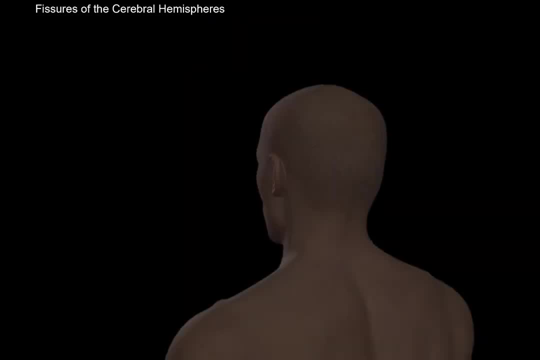 And I'll show you what I mean by this if it's unfamiliar to you, And we'll use this guy to help us illustrate this. If we take a small piece of the upper part of the skull, we'll be able to see all the 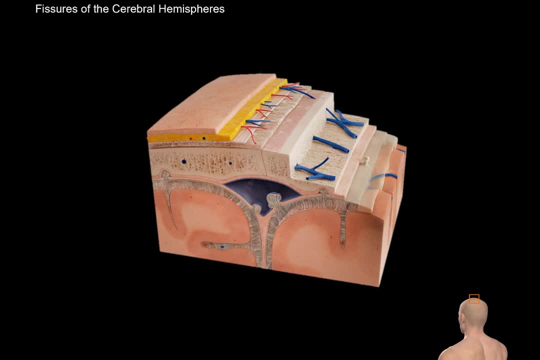 layers all the way from the skin to the brain. So the superficial part is the skin, along with all the dermal layers. Underneath the skin layers We have the skull. Directly underneath that we have the meninges And then we have our brain tissue. 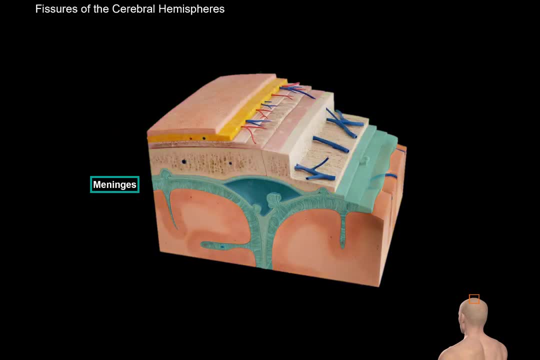 So these are the general layers, But the meninges is essentially what I want to focus on, since that is what's primarily in the cerebral fissures we talked about earlier. So the innermost meningeal layer is the pia mater, which is a delicate, thin layer of connective. 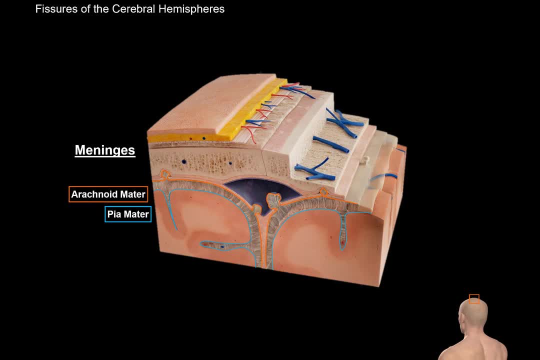 tissue. Then we have the arachnoid mater, And in between the pia mater and the arachnoid mater you'll find the subarachnoid space and you'll occasionally find these arachnoid granulations here. that pushes out the cerebrospinal. 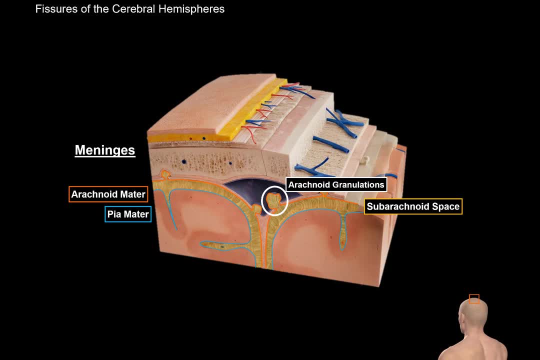 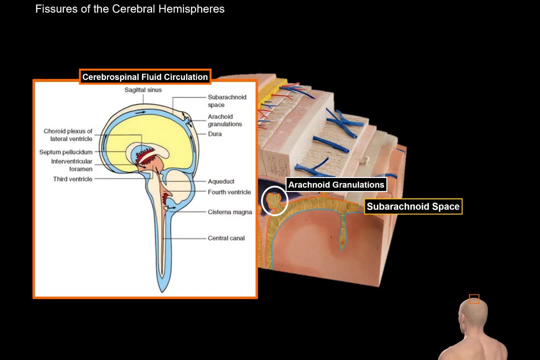 fluid from the subarachnoid space into the veins, completing the cerebrospinal fluid circulation. And here, just to quickly remind you about how the cerebrospinal fluid circulates around your brain: Cerebrospinal fluid is produced by the choroidal plexuses inside the ventricles of our brain. 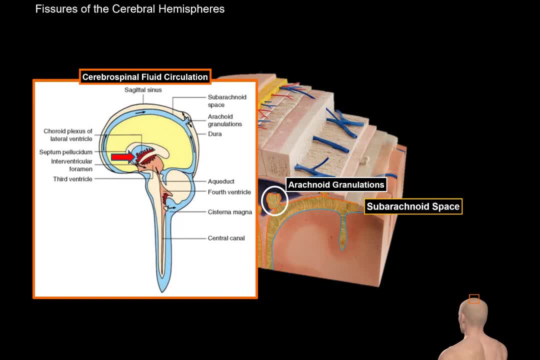 which are the lateral, third and fourth ventricles. This fluid will circulate around in the central canal and in the ventricles. This fluid is also produced in the cerebral spinal fluid and you'll notice how this fluid circulates around the central canal and the ventricles of the brain. 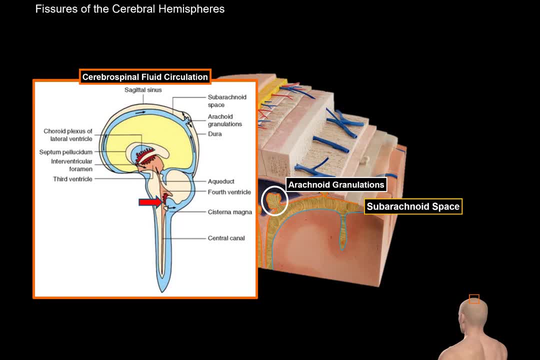 ventricles and eventually go through the lateral and medial apertures of the 4th ventricle into the subarachnoid space, which will then go through these arachnoid granulations and then into the bloodstream again. 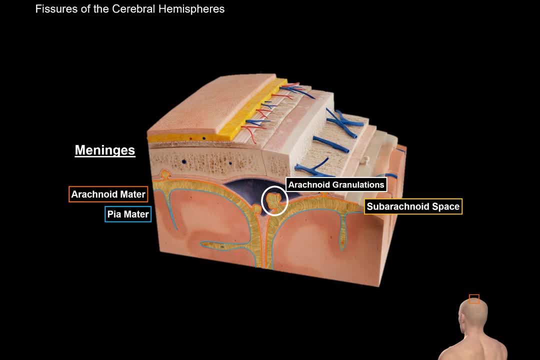 So that's the functions of the arachnoid granulations. They take the cerebrospinal fluid from the subarachnoid space and then pushes it into the dural sinuses. On top of the arachnoid mater lies the thickest of the meninges, called the dura mater. 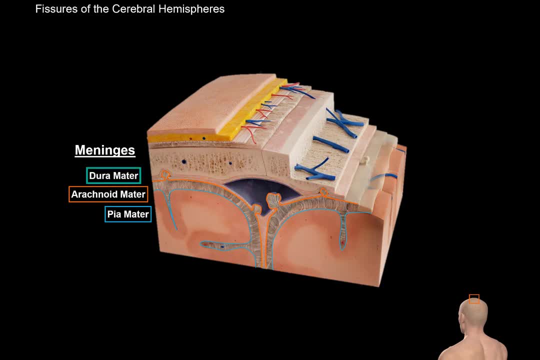 And there are two layers that make up the dura mater within our skull. There's the periosteal layer lining the internal surface of the skull, and the meningeal layer that is continuous within the brain and spinal cord. These two dural layers are bound together and only when they separate, that is when 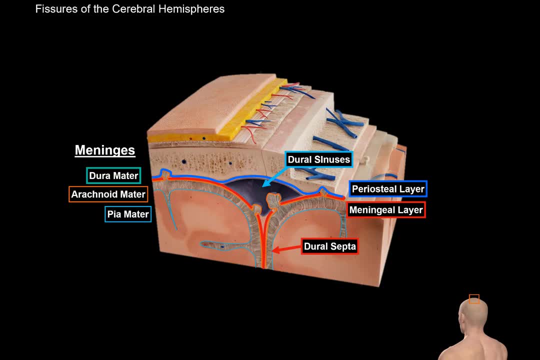 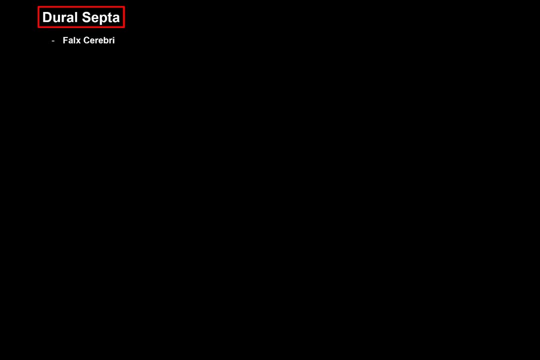 they form the dural sinuses and the dural septae. So the dural septae restricts displacement of the brain just like a seatbelt. The Falk's cerebri is the first one we're gonna talk about. So if we take the brain and cut it right about here, we'll see this. 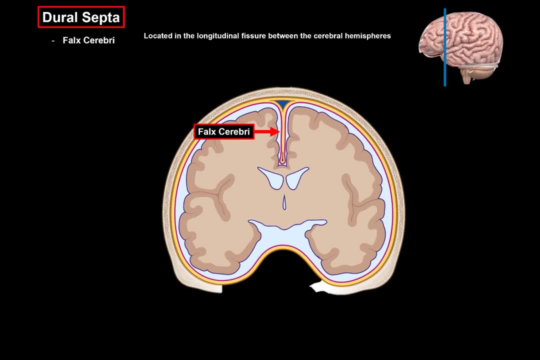 We'll see the fulcrum, The Falk's cerebri, located inside the longitudinal fissure between each cerebral hemisphere, And again, it's formed by the double layer of the meningeal part of the dural mater. Falk's means sickle like this: 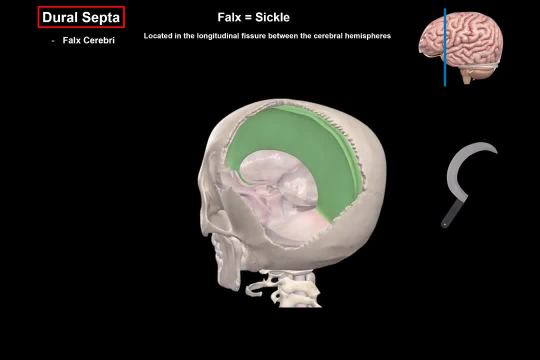 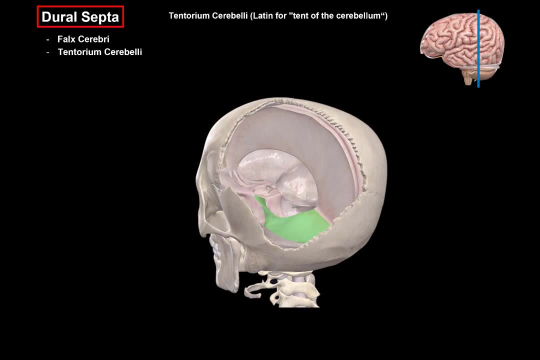 Because the Falk's cerebri is formed like a sickle within the longitudinal fissure. Then we have the Tentorium cerebelli. So if we cut the brain right about here, that's where we'll find the Tentorium cerebelli. 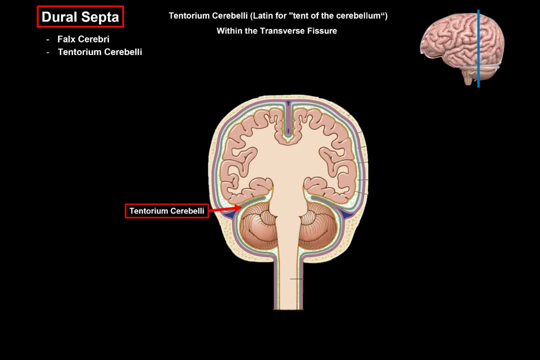 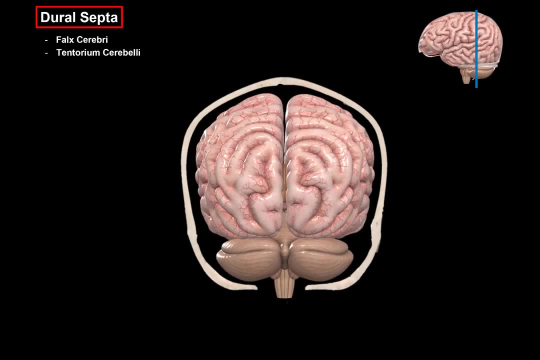 Tentorium means tent. So the Tentorium cerebelli is like a tent. It's like a tent above the cerebellum, lying within the transverse fissure of the brain. So if we take a look at this picture, the blue here is our periosteal layer of the dural. 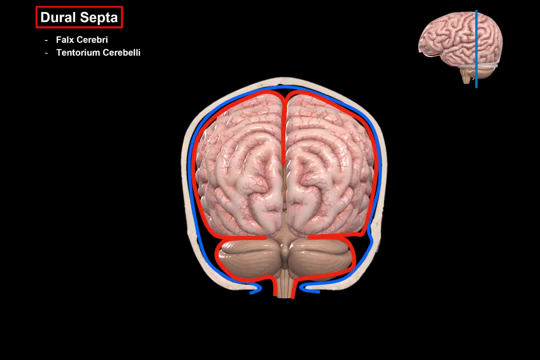 mater And in red there is the meningeal layer of the dural mater. And notice, the periosteal layer fuses at the foramen magnum and the meningeal layer goes all the way down the spinal cord. That's why there's only one dural mater layer in the spinal cord region. 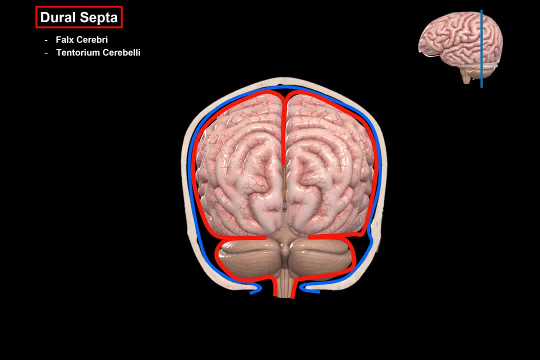 So now what we're gonna do is that we're gonna take this cross section And move it back a little bit. that's where we're going to find the Falk's cerebelli, between the two hemispheres of the cerebellum. 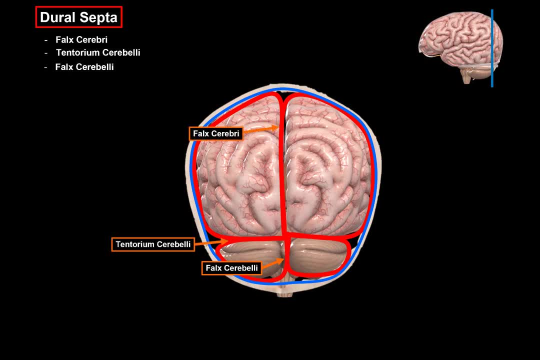 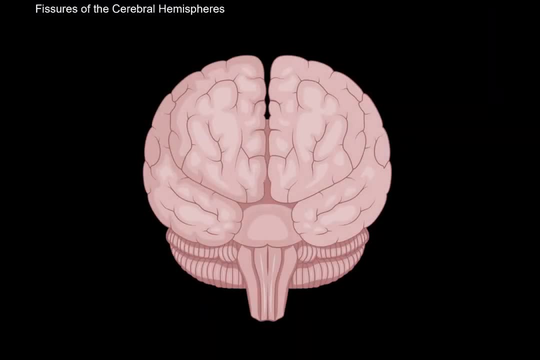 So we got the Falk's cerebri, Tentorium cerebelli and Falk's cerebelli. These are the dural septae of our brain. So if we go all the way back to the fissures, we were talking about the Falk's cerebri. 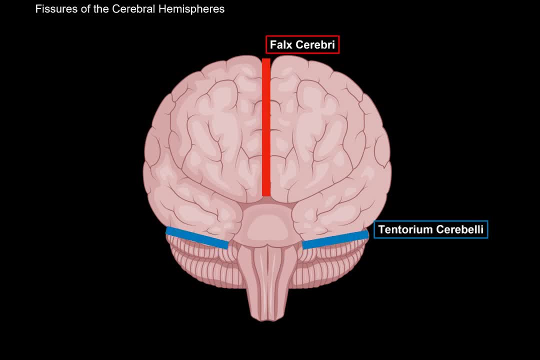 is here in the longitudinal fissure. The Tentorium cerebelli is located here in the transverse fissures of the cerebrum. So that was the surfaces and fissures of the brain. Let's now look at the lateral view to finally cover the lobes of the cerebral hemispheres. 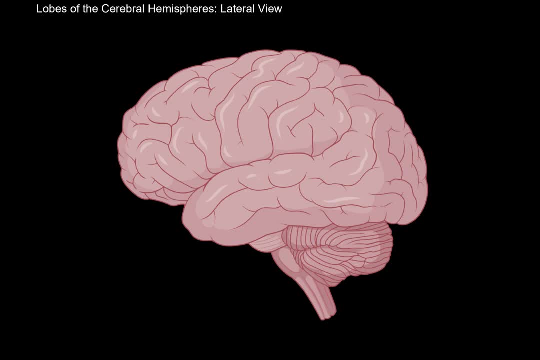 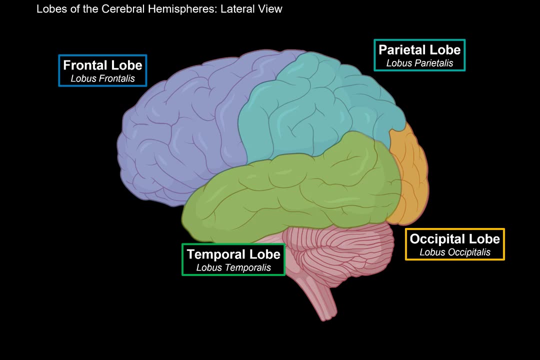 So there are 5 lobes we're gonna talk about in this video, And these are the frontal lobe, the parietal lobe, the temporal lobe and the occipital lobe. These beautiful lobes are the main large lobes on the surface of the hemispheres. 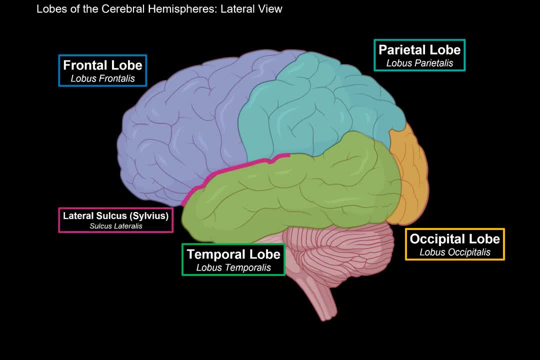 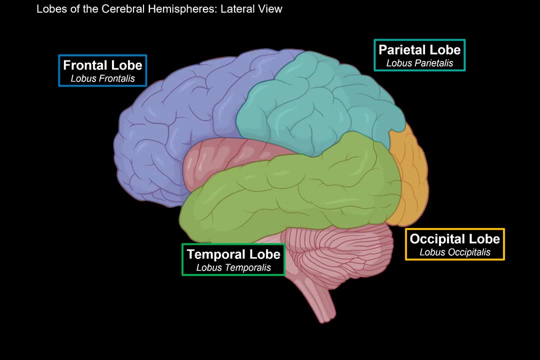 But we have a deep sulcus here between the frontal parietal and the temporal lobe, called the lateral sulcus or sulcus of sylveus. And if you would open this sulcus, You'll find one more lobe which is situated a little deeper, called the insula or insular. 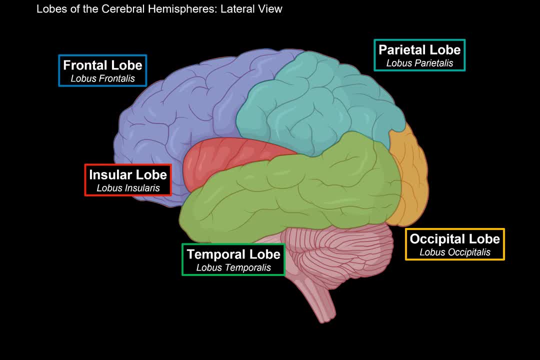 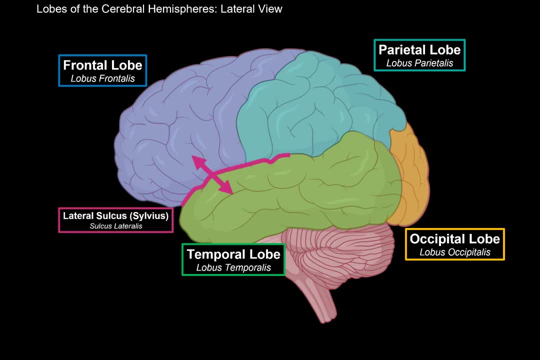 lobe. Now these lobes are separated by sulci. The first one is the sulcus. we talked about the lateral sulcus. It separates the frontal lobe from the temporal lobe and the parietal lobe from the temporal. 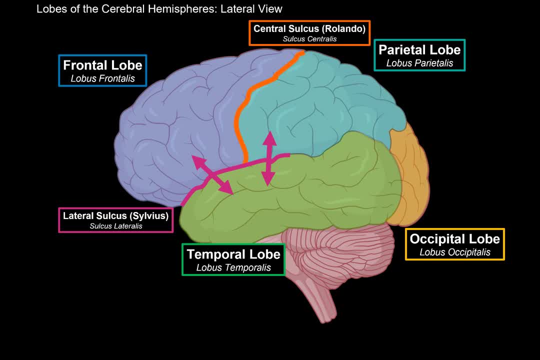 lobe. Another important sulcus we have is the central sulcus, or sometimes also referred to as the sulcus of Rolando. The central sulcus separates the frontal lobe from the parietal lobe. Another important sulcus is the parietal-occipital sulcus, separating the parietal lobe from 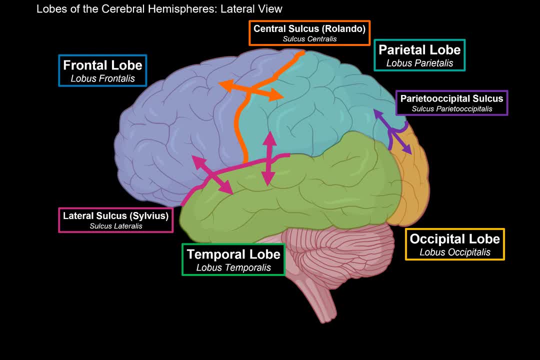 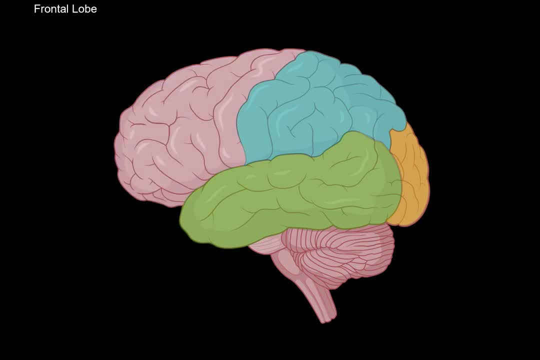 the occipital lobe. So these are the main landmarks I want you to keep in mind. Let's now cover all the gyri and sulci we'll find on the frontal lobe. The frontal lobe has a pre-central sulcus that runs parallel and in front of the central. 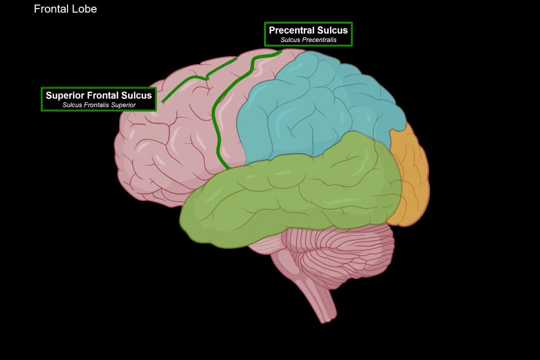 sulcus. Then there's the superior frontal sulcus and the inferior frontal sulcus. These sulci separate the brain into certain gyri. These sulci separate the brain into certain gyri. The first gyri we have is the pre-central gyrus that lies between the pre-central and 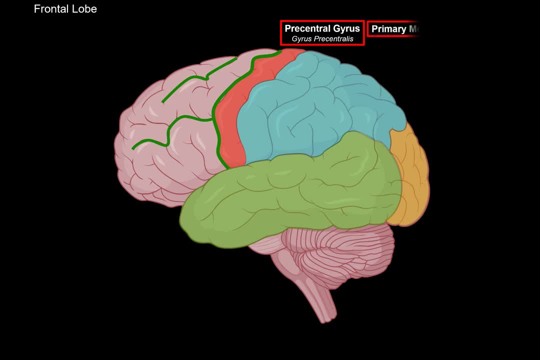 the central sulcus. The pre-central gyrus is what we call the primary motor cortex, and each segment of this gyrus is responsible for the movement of certain parts of the body. Because of this, you'll find a map of this gyrus we call the motor homunculus and it. 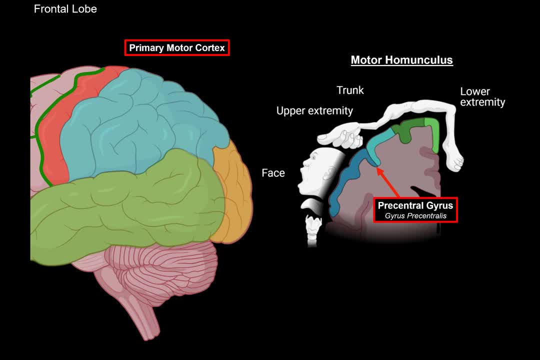 looks like this. So one part of the pre-central gyrus is responsible for the movement of the lower extremity. The other part is responsible for the movement of the upper extremity. Another part is responsible for the movement of the trunk, the upper extremity and the 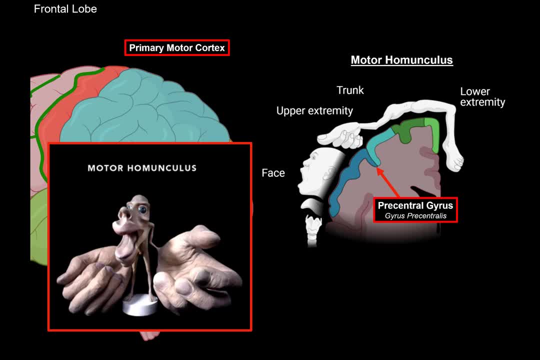 face and so on. You've probably seen this figure somewhere in your life. This figure is a distorted representation of a human body based on the neurological map of the areas and proportions of the human brain dedicated to processing motor functions of specific areas. So, for example, you see, the hands and the face are very big compared to the trunk. 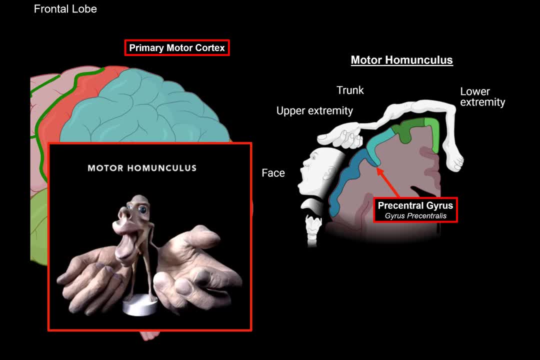 That means that a greater portion of the pre-central gyrus lies between the pre-central gyrus and the central sulcus. So the pre-central gyrus is dedicated for these areas. And again, which layer of the cerebral cortex do these tracts come from? 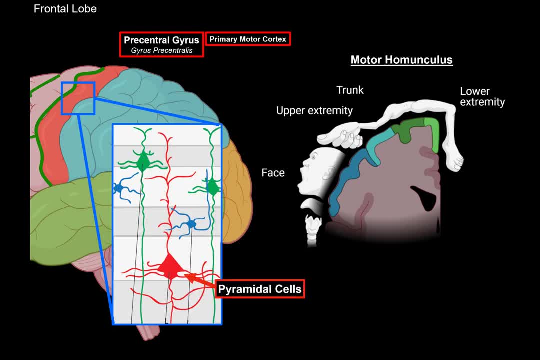 The tracts come from the pyramidal cells of the internal pyramidal layer. These tracts are what we call pyramidal tracts that give off voluntary movements. They are the corticospinal tract and the corticonuclear tract. 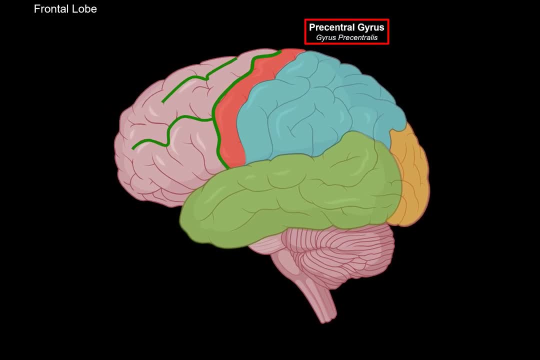 So that is the pre-central gyrus. Now, above the superior frontal sulcus lie the superior frontal gyrus, Between the superior and the inferior frontal sulcus lies the middle frontal gyrus, And below the inferior frontal sulcus lie the inferior frontal gyrus. 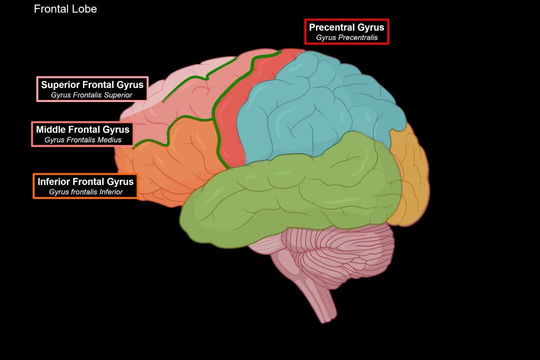 These gyri are referred to as the pre-frontal cortex and have association areas that make up our personality. On the inferior frontal gyrus you'll find an area called the Broca's area, which is the motor speech center. It is involved in language speech production and comprehension. 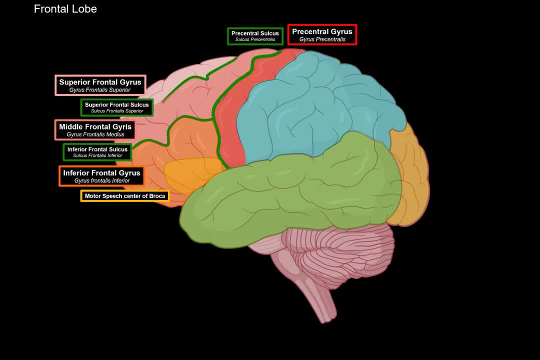 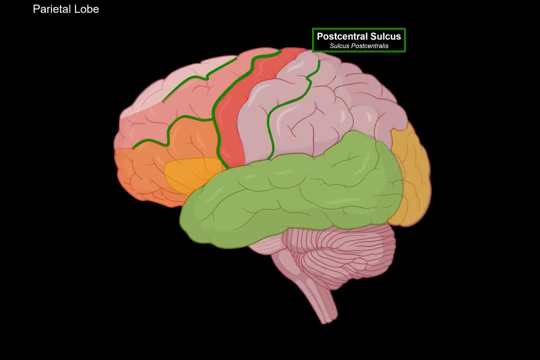 So what is it? That was all the gyri and sulci of the frontal cortex from a lateral view. Now let's see the parietal lobe. The parietal lobe has a post-central sulcus. It's post because it lies after the central sulcus. 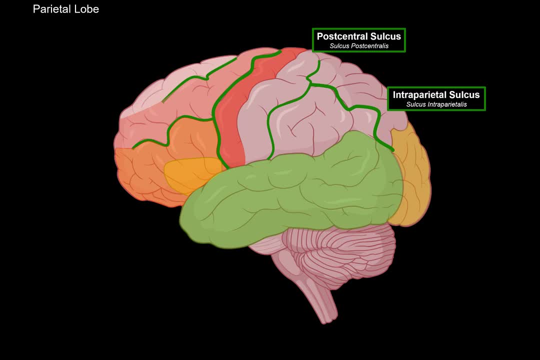 Then there's the intraparietal sulcus separating the parietal lobe into two lobules. Alright, let's see the gyri. Here we'll find the post-central gyrus, which is the primary somatosensory cortex. 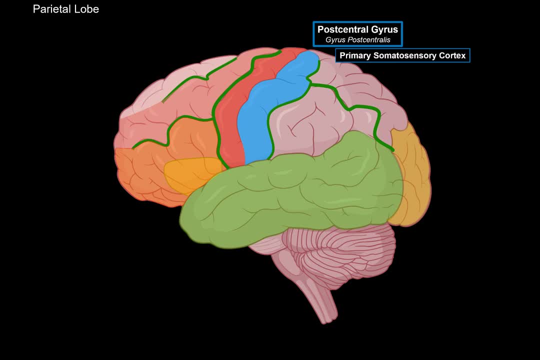 And that again receives sensory information. We can get information regarding touch, pain, temperature and proper reception, which is basically the position of the different body parts And again, just like the pre-central gyrus, you can draw a map of the post-central gyrus. 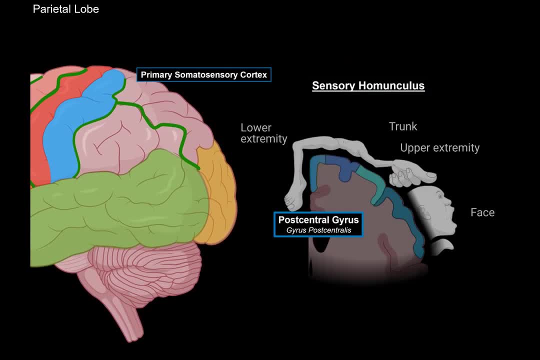 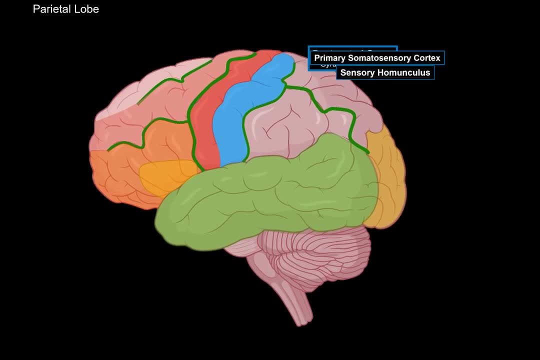 as well Calling it the sensory homunculus, which basically also have different regions receiving different sensations from different areas of the body. So that is the post central gyrus. The intraparietal sulcus divides the parietal lobe into two lobules. 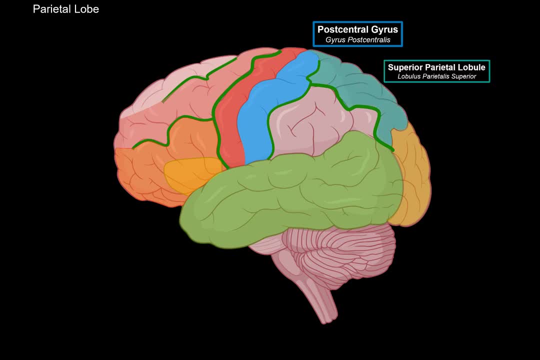 The spina bianca offers a pathogen rundown of the central lobes. The central lobe also has sensors. Superior to the intraparietal sulcus lies the superior parietal lobule, which is an association area of the brain. 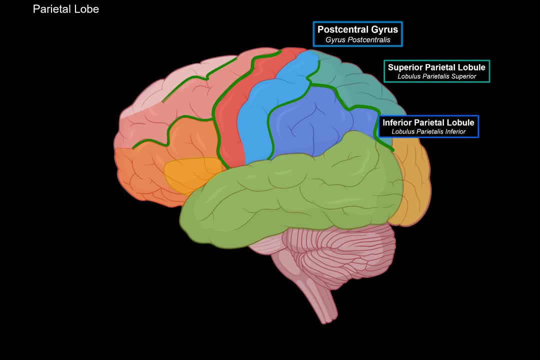 And below the intraparietal sulcus lies the inferior parietal lobule, which is also a sensory association area. But here you'll find two gyri. you'll find the supramarginal gyri lying above the end of the lateral sulcus, and the angular gyrus, which is the reading center of the. 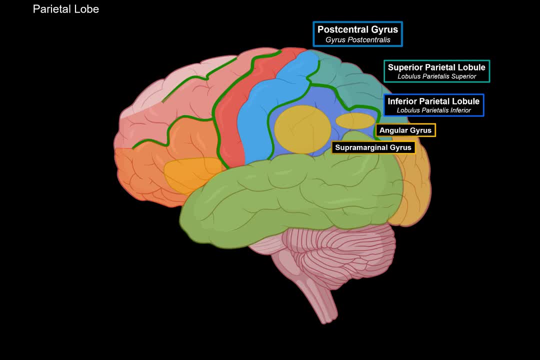 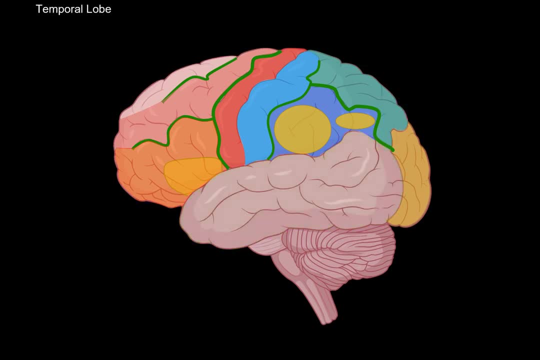 brain. This area gives us the possibility to understand written words and metaphors. So that is the parietal lobe. Next we have the temporal lobe, And the temporal lobe has the superior temporal sulcus and the inferior temporal sulcus. 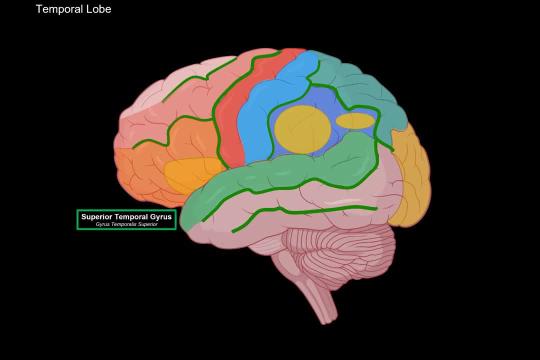 And they divide the temporal lobe into three gyri. First we have the superior temporal gyrus. Here you'll find the primary auditory cortex that receives auditory information. Now, where did these neurons come from? They come from the cochlea, Through the cochlear nerve. 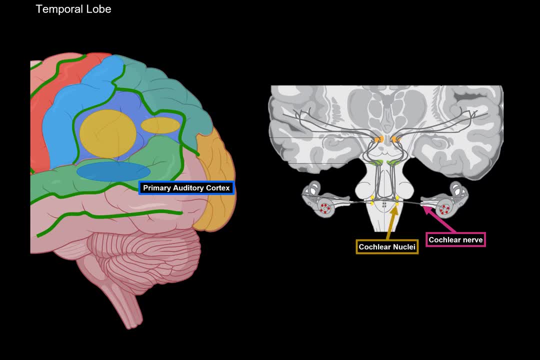 This nerve will synapse with the cochlear nuclei, then cross and form the trapezoid body of Pons. Then they will ascend as the lateral lemniscus and synapse with the inferior colliculus And then, through the brachium of the inferior colliculus, they will go to the medial geniculate. 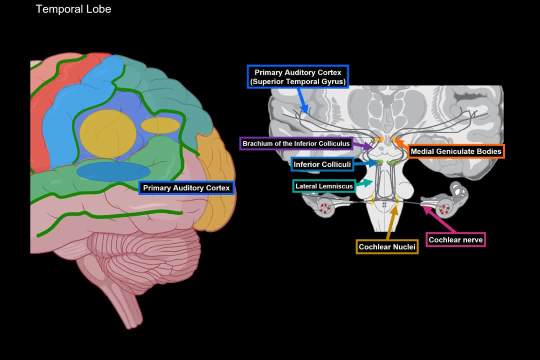 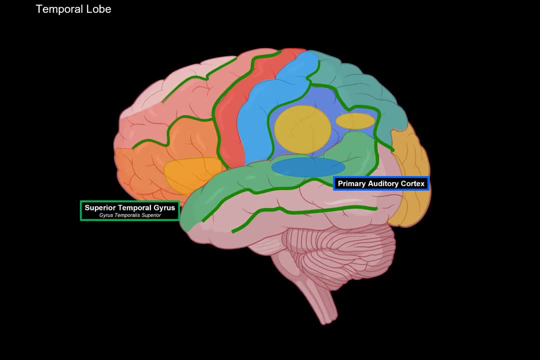 body of the diencephalon and then finally go to the nuclei of the primary auditory cortex, which is here at the superior temporal gyrus. And when they get here, you're consciously aware of the things you're hearing. And when they get here, you're consciously aware of the things you're hearing. 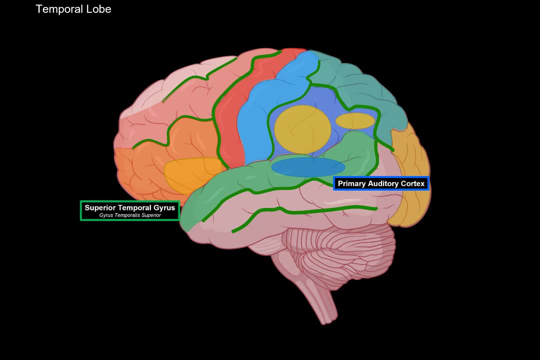 And when they get here, you're consciously aware of the things you're hearing. Another area you'll find on the superior temporal gyrus is the Wernicke's area, which is a sensory area of speech In unfortunate situations where people receive a direct hit on the temporal side of the head. 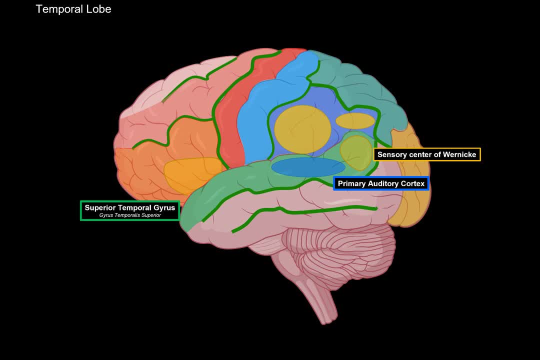 this area might get damaged. And then the patient shows a condition called receptive aphasia, where their speech appears normal grammatically but there's no meaning in what they're saying. So, for example, if they want to say I'm going to the house, they will say I am walking. 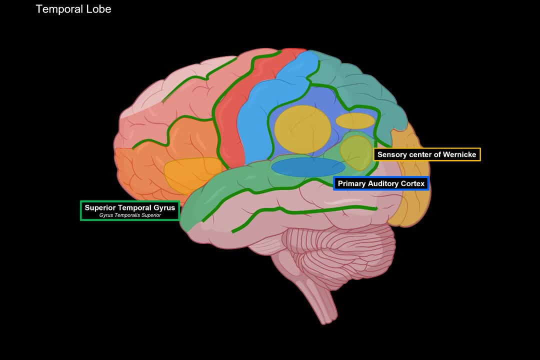 a head horse to the ice cream. There's literally no sense in the words they're saying, but their speech appeared normal grammatically. So this area is crucial for speech And that is the superior temporal gyrus. Then we have the middle temporal gyrus and the inferior temporal gyrus, which are association. 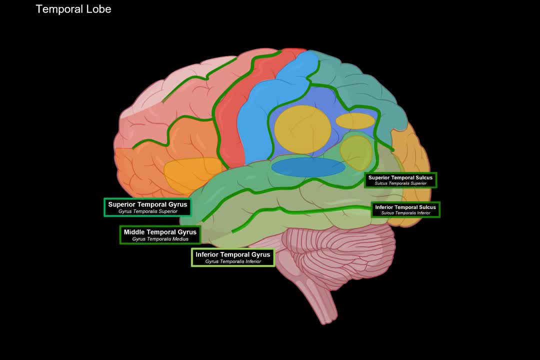 areas as well. So that is the temporal lobe. Next let's do the occipital lobe. There's not much to say about this lobe from this perspective, as you're only seeing a small portion of it, But if we turn this image to the other side, we can look at the medial surface of the cerebral. 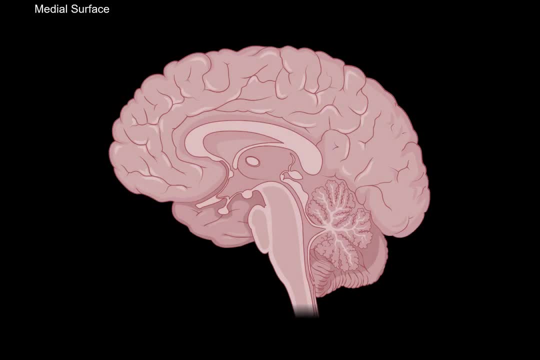 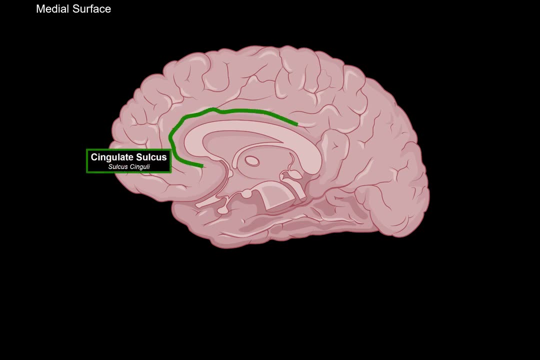 hemispheres. Let's now focus on the gyri and sulci we'll find in this area. So let's remove the brainstem so that we can see as much of the cortex as possible. So, first off, we have a deep fissure here we call the cingular sulcus. 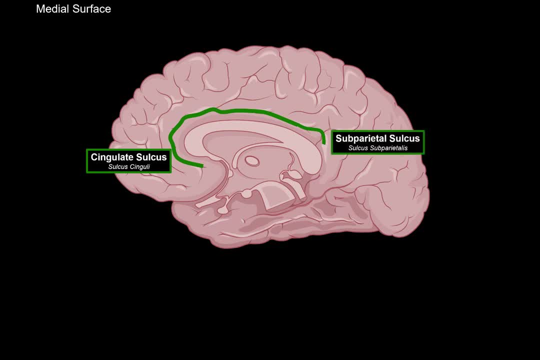 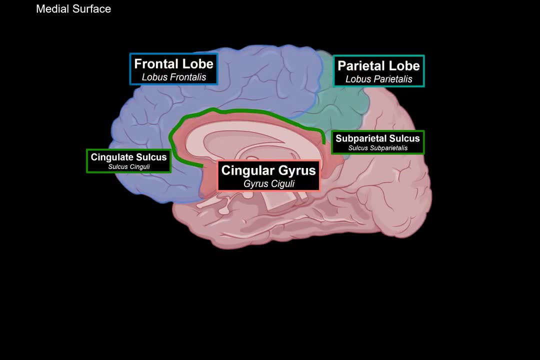 This sulcus continues backwards and eventually becomes the subparietal sulcus, And what the sulcus does is that it separates the frontal lobe and the parietal lobe from the cingulate gyrus. The cingulate gyrus is a part of the limbic system, which is a system responsible for. 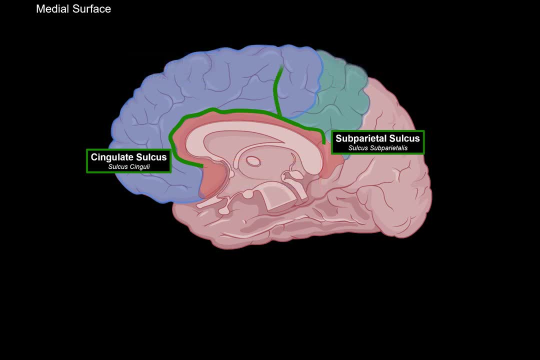 processing emotions and behaviour regulation. Then we have the paracentral sulcus and the marginal sulcus, And in between them there's an area we call the paracentral gyrus, which is a part of the precentral and postcentral gyrus. 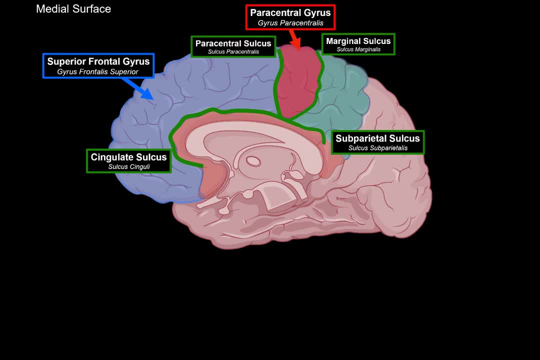 The majority of the frontal lobe. the blue area you see here is a part of the superior frontal gyrus which we looked at earlier. Then, if we shift our focus to the posterior side, We'll find the parieto-occipital sulcus which, remember, is the landmark between the 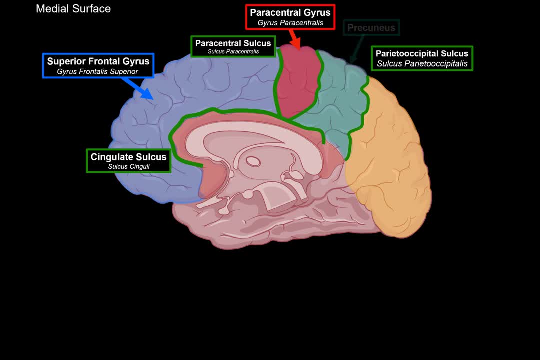 parietal lobe and the occipital lobe. In front of the parieto-occipital sulcus there's the precuneus, which is an association area located in the parietal lobe. But behind the parieto-occipital sulcus you'll find the cuneus, which is a part of the occipital 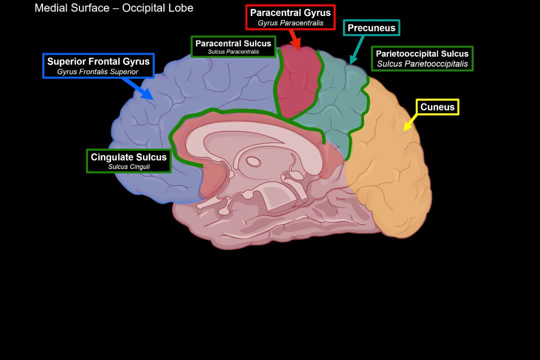 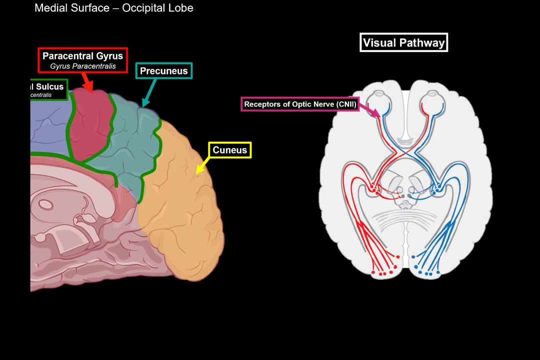 lobe, The cuneus, contains the primary and the secondary visual cortex, So let's go through the visual pathway again. On the retina of the eyeball we have receptors for the optic nerve, the second cranial nerve that leaves the eyeballs. 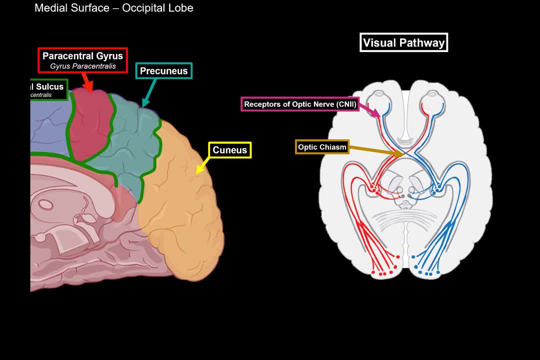 Half of these tracts will cross to the other side and form the optic chiasm. Then they will synapse with the lateral geniculate bodies and then go to the primary visual cortex, which is the cuneus of the occipital lobe. 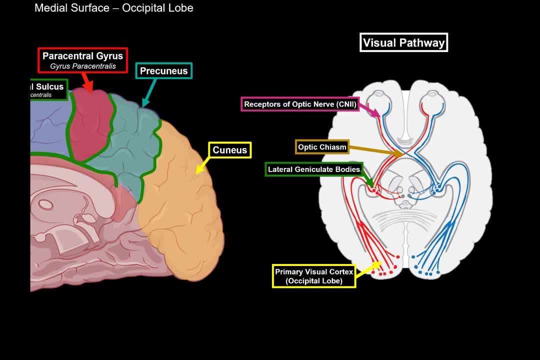 When the nerve goes to the primary visual cortex, that is when we're consciously aware of what the eyes perceive. These fibers can also go to the superior colliculi of the midline. They will simply move in and out and then go over there, so that action is perfectly. 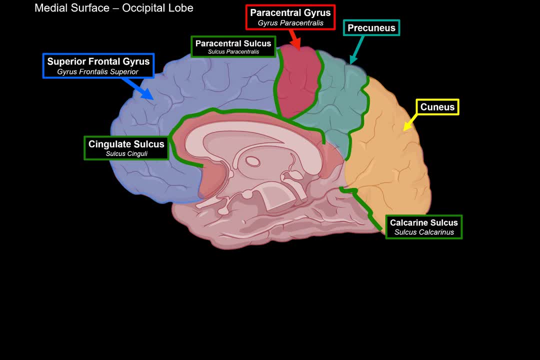 visible While we're on the command. behind the tutteleus it arms both limbs to, in this case, the wide Broadway, and then many more fibers come into contact with the lower RICHARD, open up to the palate ofорic rose. This can also be done with the pancarapsas, which is the part of the occipital lobe that 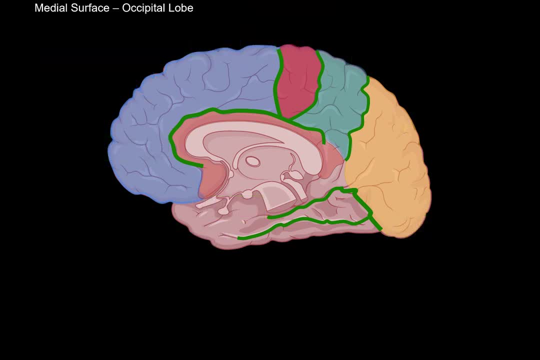 supports the temporal lobe so that move inside and out of the temporal lobe. The collateral sulcus separates the lateral occipital temporal gyrus from the medial occipital temporal gyrus and the parahippocampal gyrus. 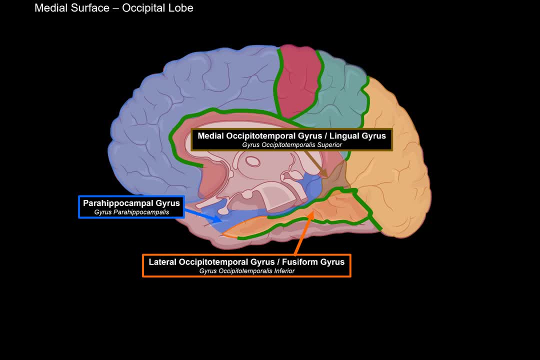 These are the pacing lobes. They're unconnected occipitotemporal gyrus is sometimes referred to as the fusiform gyrus. The medial occipitotemporal gyrus is sometimes referred to as the lingual gyrus. 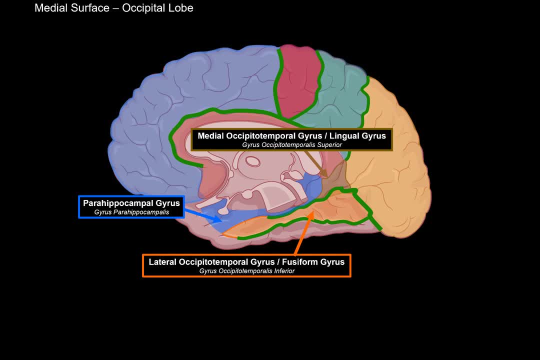 And these two areas are what we call the visual association areas, So they take in information from the primary visual cortex and they give you the possibility to take past experiences, let's say someone's face, or maybe even a flower or a facial expression. 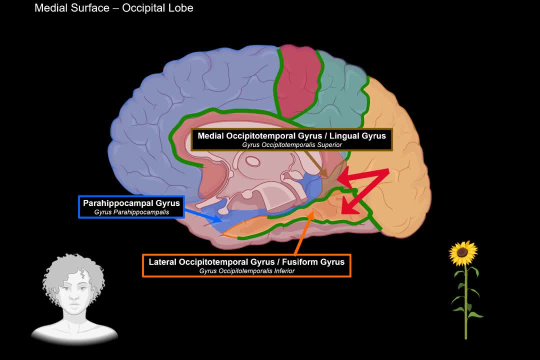 and it helps with recognition. It gives meaning to the image you're seeing. So the cuneus, the lateral occipitotemporal gyrus and the medial occipitotemporal gyrus are all a part of the occipital lobe. 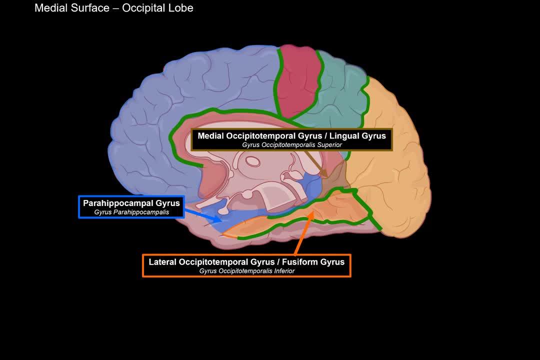 Awesome. The parahippocampal gyrus is kind of a continuation of the cingulate gyrus, so it's also a part of the limbic system. Lastly, the gyrus down here is the inferior temporal gyrus we talked about earlier. 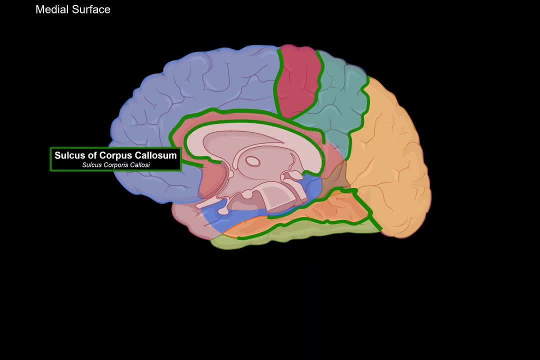 So that's these. What other structures do we see here? We have the sulcus of the corpus callosum- We'll talk about that later- The corpus callosum which divides the cingulate gyrus from the corpus callosum. 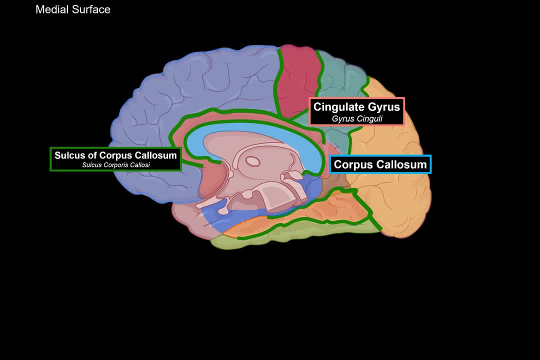 The corpus callosum itself doesn't really have any actual function. however, it's a really important part of the brain because it contains a lot of fibers that connect both hemispheres. That's really what it does: It just has fibers that go from the left hemisphere to the right hemisphere and vice versa. 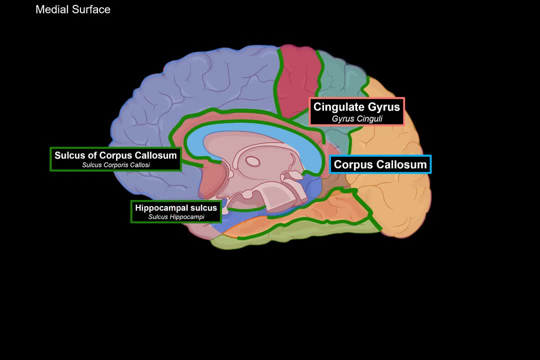 Now, another sulcus we can find is the hippocampal sulcus, And that's a sulcus that divides the parahippocampal gyrus from the dentate gyrus. Again, this is a very important part. The parahippocampal gyrus is a part of the hippocampal sulcus and it's the part that 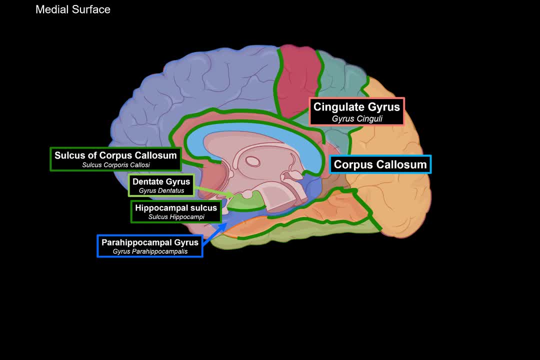 divides the parahippocampal gyrus from the dentate gyrus gyrus. The dentate gyrus is a part of the hippocampus which we'll talk about in the next video and it contributes to forming new memory. Now, from the parahippocampal gyrus it's going 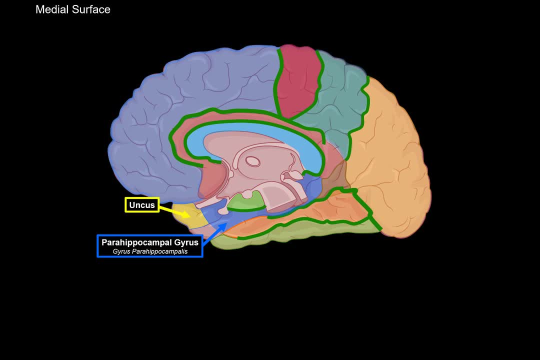 to continue as the uncus, and the uncus is a hook-like structure that is a part of the olfactory cortex receiving information about smell. The last thing I wanna mention here on the medial surface is a narrowing that is associated with the cingulate gyrus and that is the isthmus of 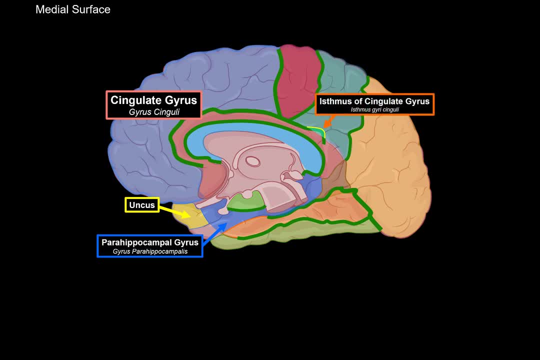 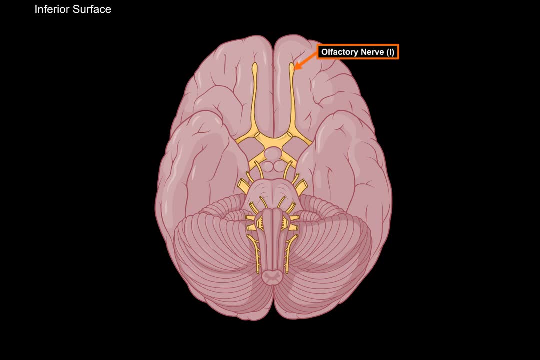 the cingulate gyrus, which is located here in this area. So that was all the structures on the medial surface. Now, if we look at the inferior view of the brain, we'll find the olfactory nerve, which is the cranial nerve number one, and the optic chiasm of the optic tract. 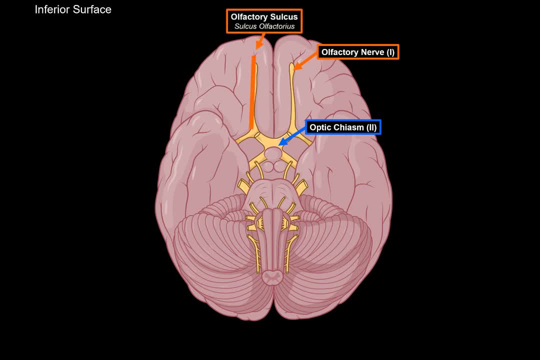 The olfactory nerve lies on a sulcus called the olfactory sulcus, And the olfactory sulcus divides the lower surface of the frontal lobe into two parts. It divides it into the gyrus rectus, which is a part of the frontal lobe, and the gyrus rectus, which is a part of the frontal lobe. 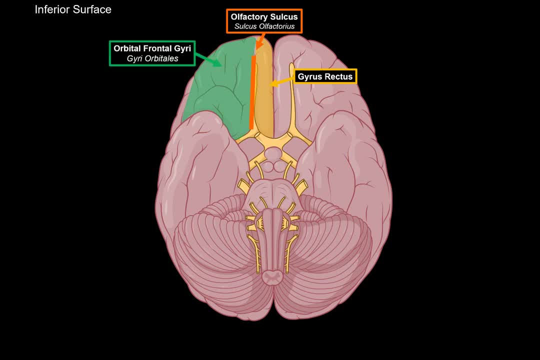 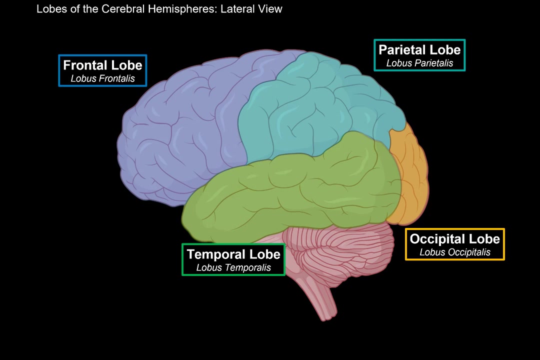 And the orbital frontal gyrus, or gyrus orbitalis, which is also a part of the prefrontal cortex. On this gyrus you'll find many small sulci called the orbital sulci or orbital frontal sulci. So that was all of these lobes. Lastly, let's open up the lateral 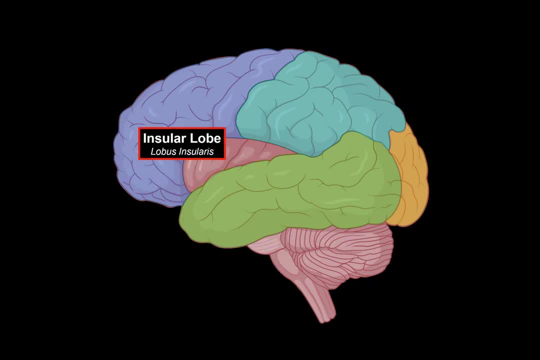 sulcus and talk about the insular lobe. Now, what I want you guys to know about the insula are two things. One is that it's divided into the short gyrus of insula and the long gyrus of insula, And two is that the insula is responsible for receiving taste sensation. 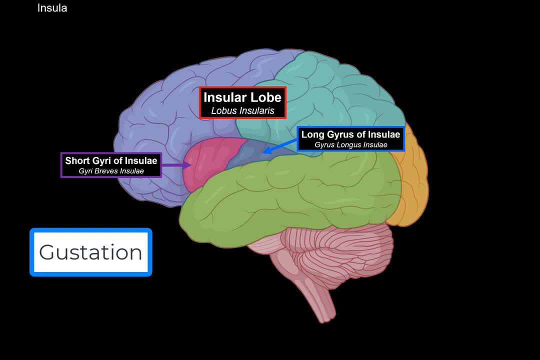 so gustation. The insula is what we call the gustation cortex, because it perceives taste. It tells us what kind of taste it is: if it's sweet, if it's sour, if it's bitter, if it's salty, if it's umami. The other function of the insula is visceral sensation. So sensation. 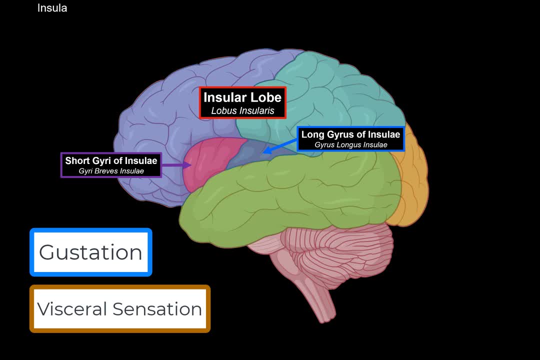 comes from the GI tract, the heart, the lungs. If a person has gastroenteritis, the pain from that GI tract will go to the insula and make you aware of that. The last function is that it's believed that this may be where your vestibular cortex is located, And the vestibular cortex would be. 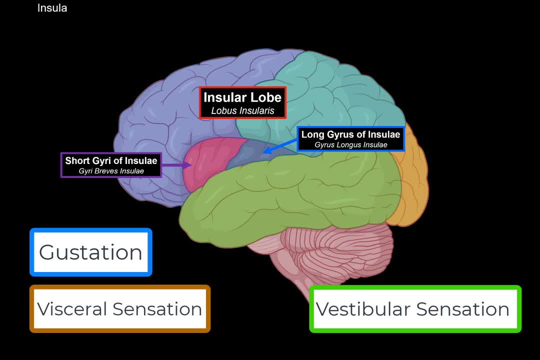 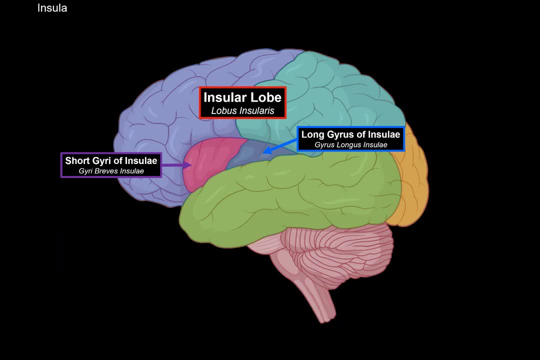 involved in your vestibular sensation, which is basically your sense of movement. So static equilibrium and rotational acceleration and all of those things may go to the insula. Alright, guys, so that was a video about the cerebral cortex. If you found this video helpful.